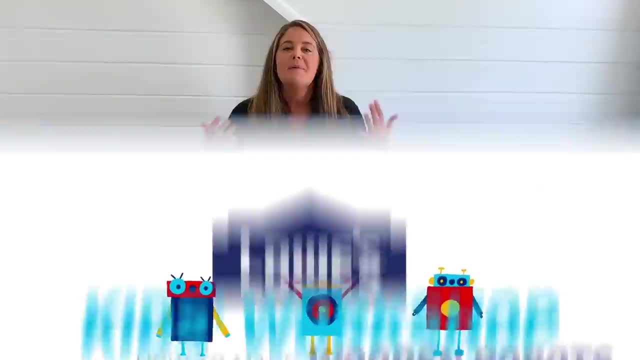 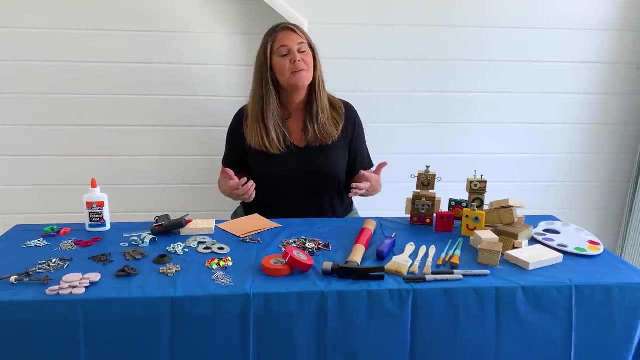 Hey friends, Monica here. Whenever you and your kids are home, whether it be for a long weekend, a vacation or even a snow day, it doesn't take very long until you hear the classic I'm bored. We've all heard it and we've probably said it as kids too. As a DIY, loving mom of four, 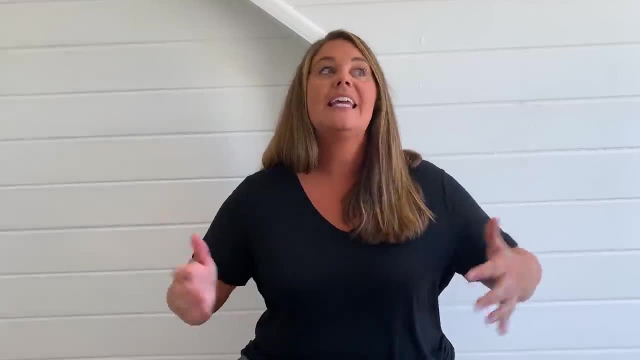 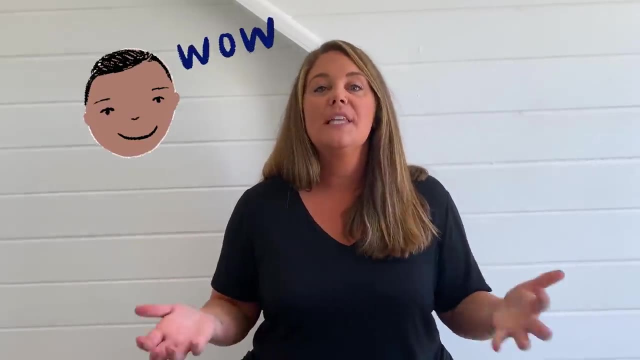 I have tried all kinds of creative activities to keep my kids engaged and entertained, And I'm going to share some of my very favorite projects with you. These are all kid approved and ones that we really enjoy doing together, And I think you will too. Let's get started. 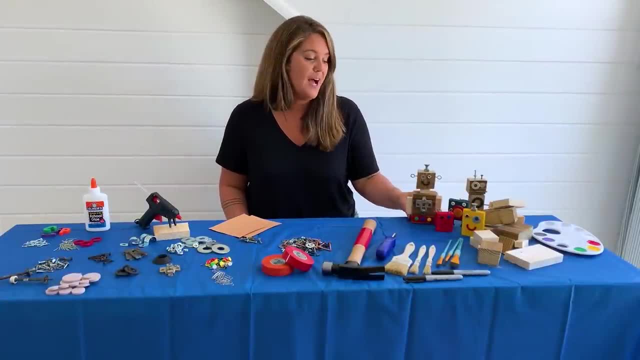 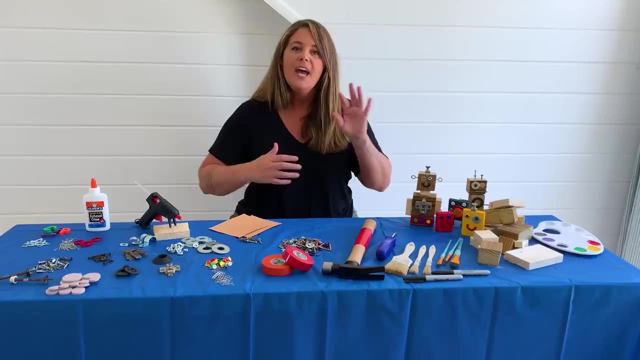 Today we are going to make some wooden robots. These are an awesome project that you can make with your kids. I love it because it totally unleashes their creativity, And I think this is a project that works really well for a wide age range. There's just a million reasons why. 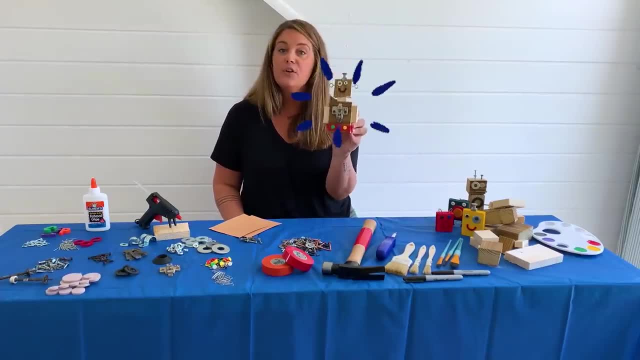 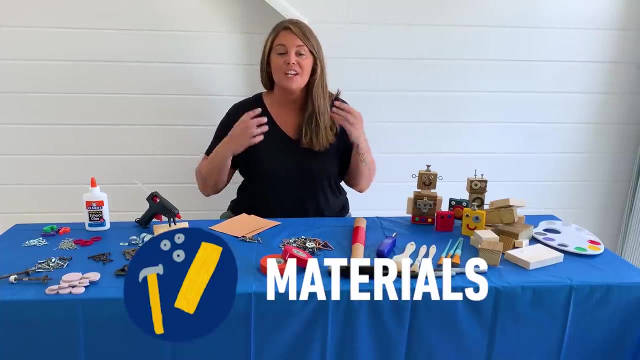 I like this. Probably the number one reason is that they're so stinking cute. I feel like they're just maybe one of the cutest crafts you'll ever do. As far as materials go, this is very much a scrap project. You're going to use a lot of leftover items that you have in. 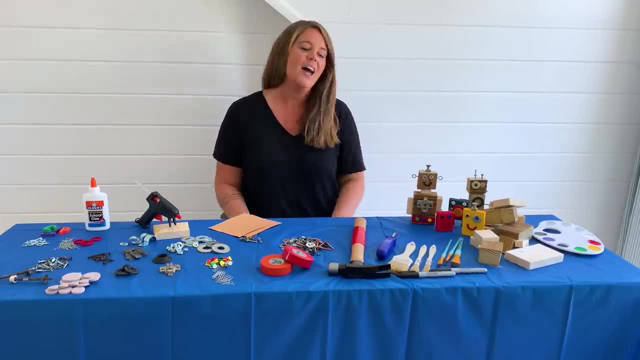 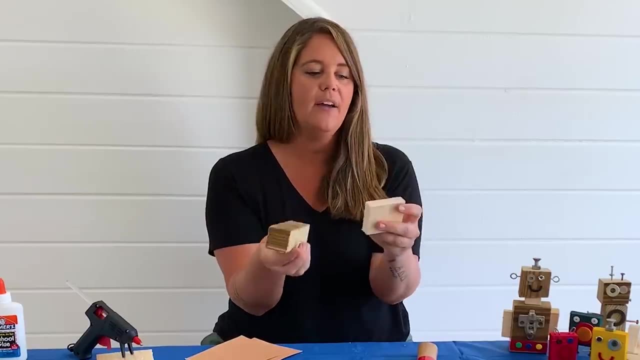 your garage. hopefully from other DIY projects, we've inspired you to try A couple essentials. you are definitely going to want to make sure that you have some wood scraps. Now, what I've done here is I just, anytime I'm done with a project, kind of keep pieces around. I 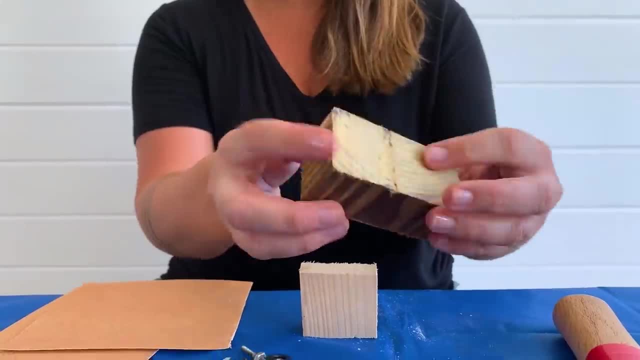 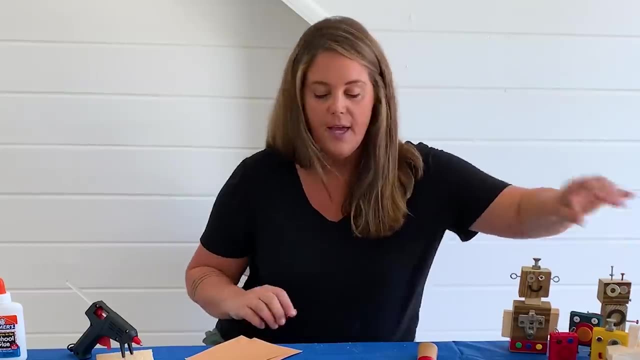 keep them larger, and I just chopped these down. These are all completely raw from my scrap bin. None of them have been sanded down yet, So that's going to be the second thing you need. You need wood and you want to have sandpaper, And this was just a regular sheet that I cut down. 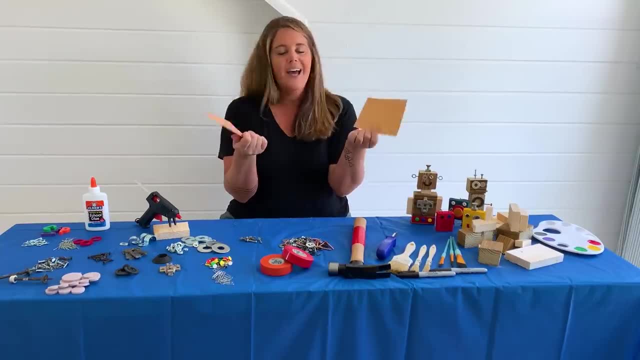 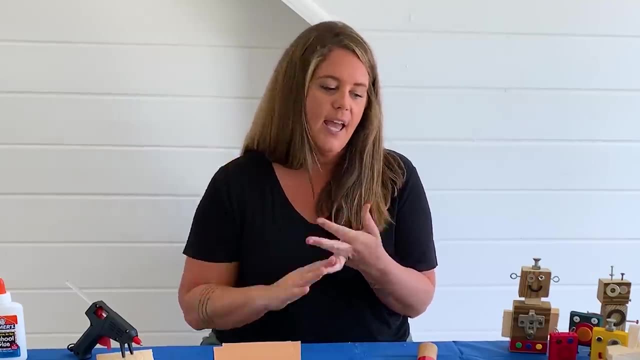 When I'm working with my kids, I like to give them a little piece of sandpaper each. I just think it's easier for them to work with and manage and it wastes a little bit less. I recommend having a hammer and a screwdriver Now. this has both flathead and Phillips. 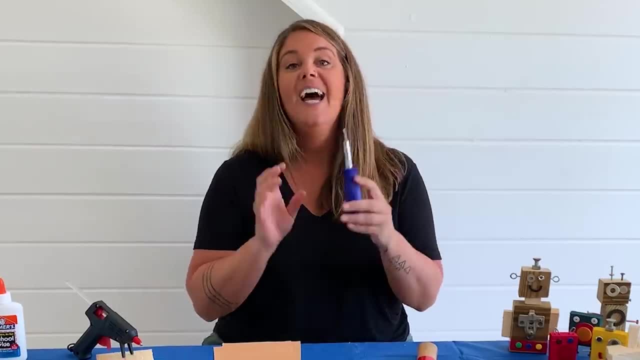 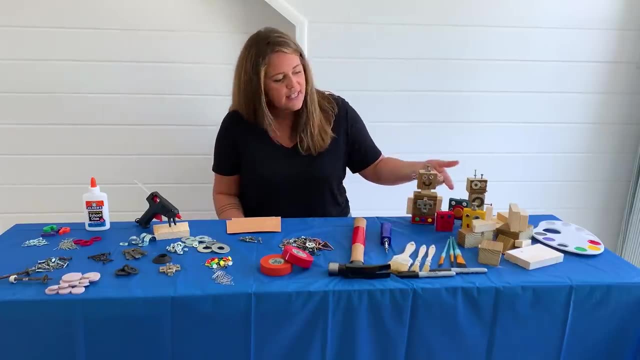 and I can switch it back and forth, because I have quite a variety of screws and nuts and bolts and things that I'm going to use on these robots. I also have some paint brushes If you want to paint your robots. I think the painted ones are really, really cute. 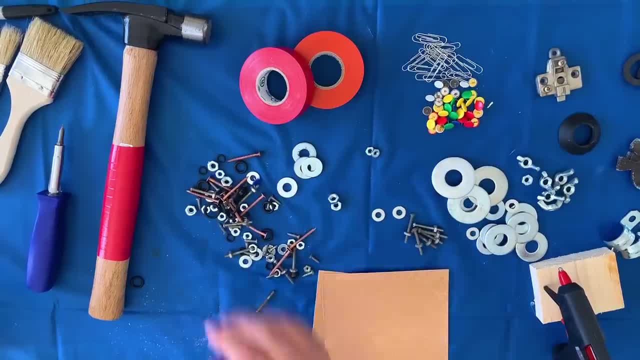 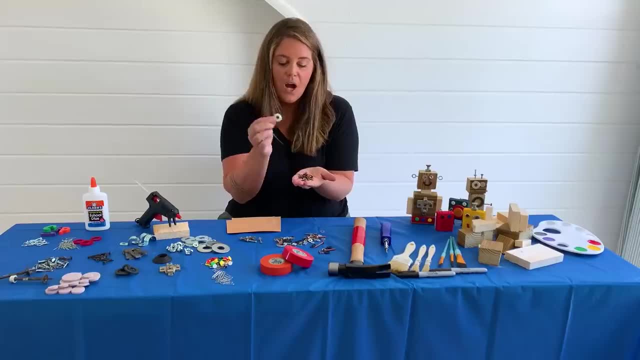 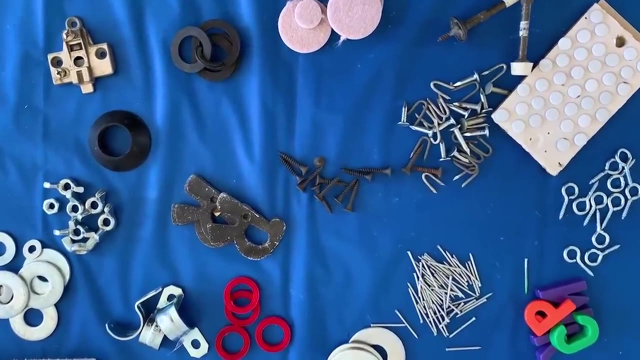 Now it comes to the good stuff. This is where all the cute little accessories come from. So I went into the garage and I just grabbed a huge assortment of screws and nails and washers and rubber washers and wing nuts. Really anything can become part of a robot. One thing that I 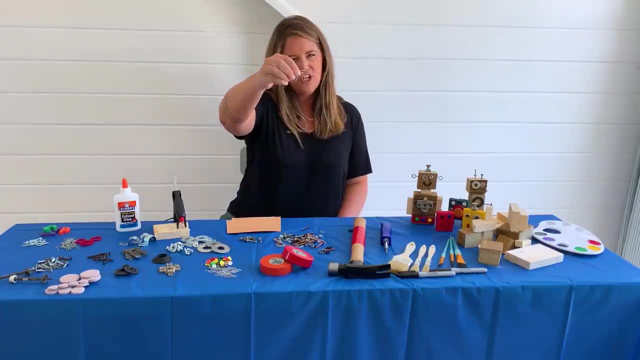 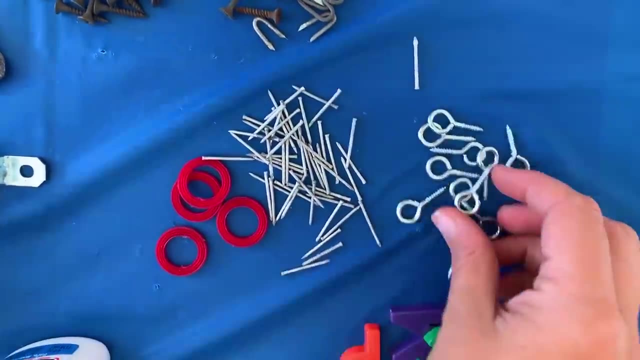 definitely would recommend are some very small little finishing nails. They're really helpful, especially if you have older kids, because then you can make certain parts of your robot. It's kind of functional. And then also eye hooks are really adorable for antlers and for ears and 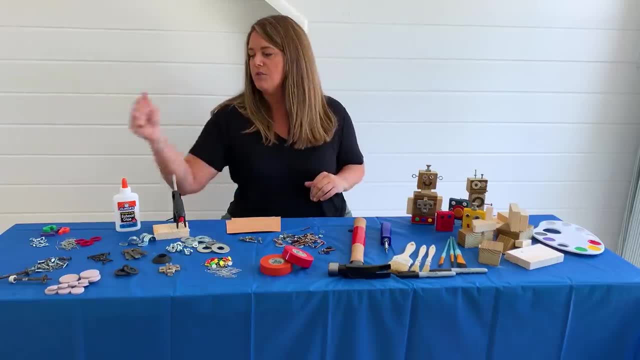 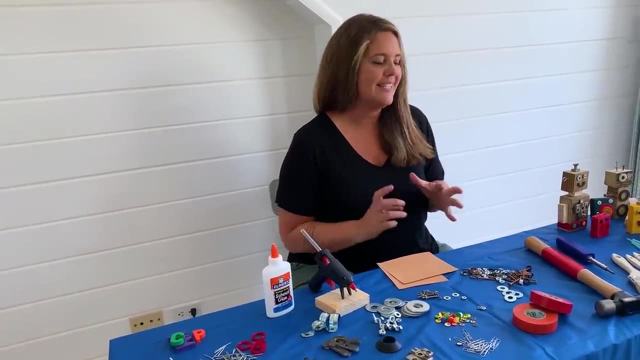 all kinds of things. I guess they're called antennas. Eye hooks are really great too. Those will come in handy All right. after you've gotten your materials, it is time to move on to step one, which is choosing wood and sanding it down. I kind of like rectangle pieces And again. 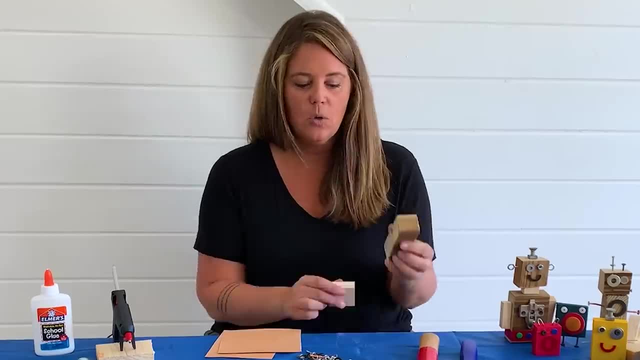 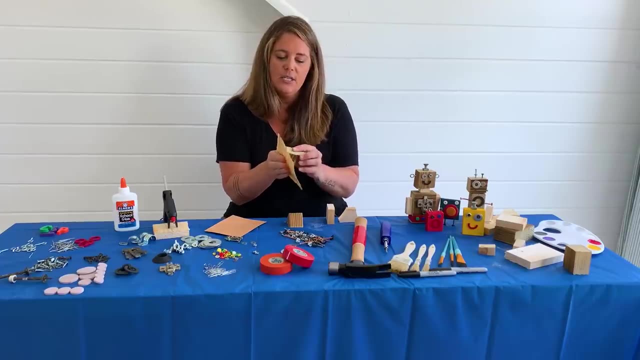 they don't have to be perfect. This is not a perfect square, and that's totally okay. What I have here is some 120 grit sandpaper. It's going to just kind of work the edges here without doing too much. Once you have your pieces for a robot all sanded down, you have a couple options here. 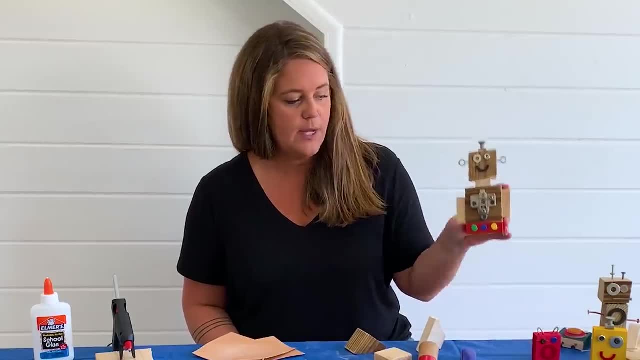 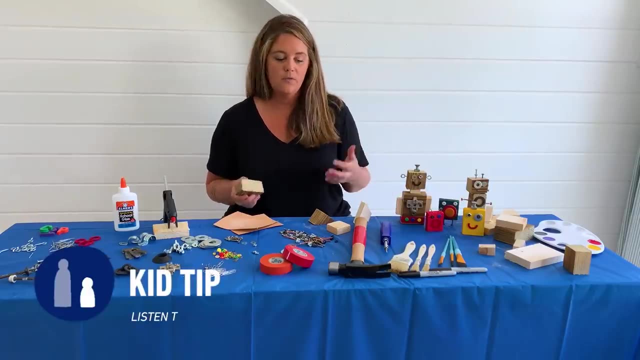 You can go with a natural looking robot, like we did for these ones, or you can go with some painted robots, like we did for these little guys in front. If you were going to do a painted robot, now would be the time to start painting, because you'd want to paint your wood, get it dry and then come back. 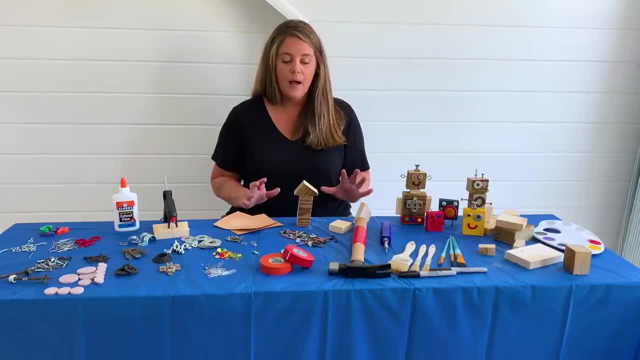 to materials. Let me talk to you about how to assemble your robot. A couple options here. You could go with straight school glue. That's an okay option if you have younger kids. The only tricky part to that is you need to build your robot laying flat. They're kind of just going to need to stick items. 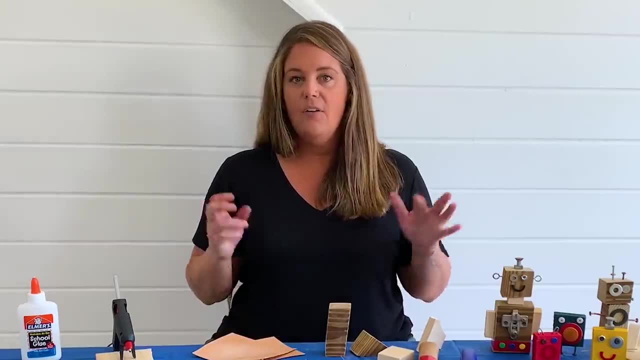 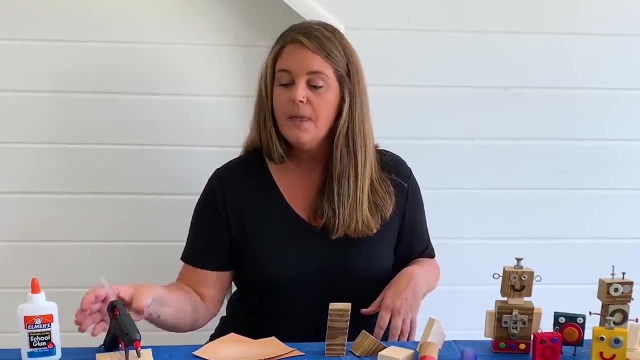 on and let it dry, because it does take a little while. If you have older kids, you could consider using a glue gun, or maybe have the parent use a glue gun. The kids decide where it wants to go, And then again, if you have older kids, some of these parts can actually 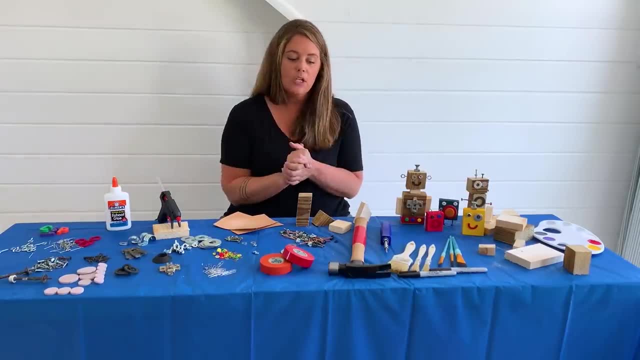 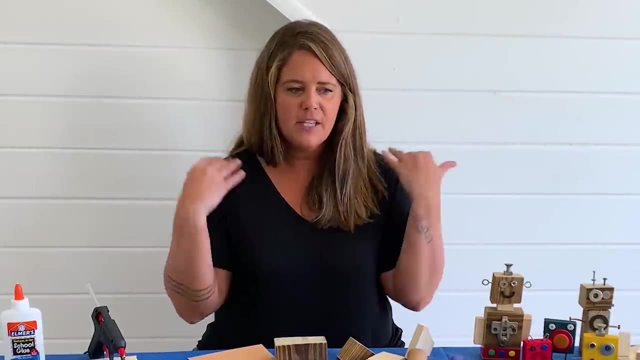 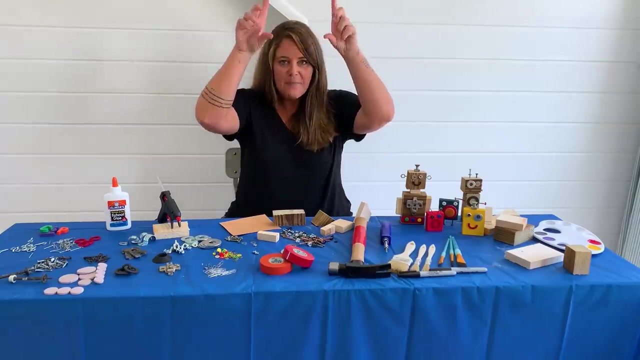 get screwed and nailed right onto the robot. So I'm going to do a combination of hot glue and nailing and screwing for mine All right. now it's time to get creative, And you have to think about what does a robot have? It has a body, it has arms, it has legs, it could have antenna coming out of. 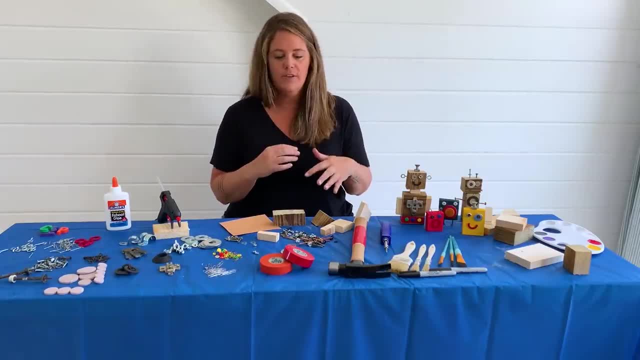 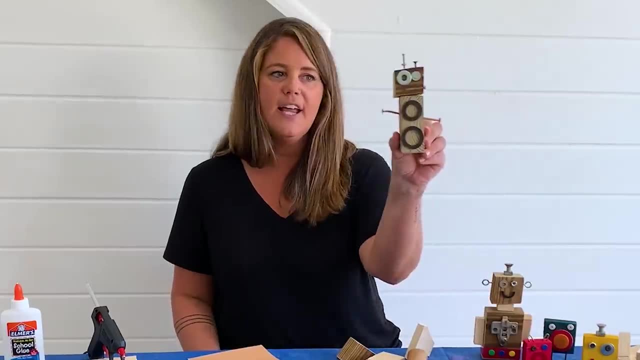 it. So really, all of these pieces could almost function for a variety of different parts, And what I'm going to do first is start by adding some arms to my guy, And I really like the way the little bent nail looks on this fella, So I'm going to try that for you. So I have these. 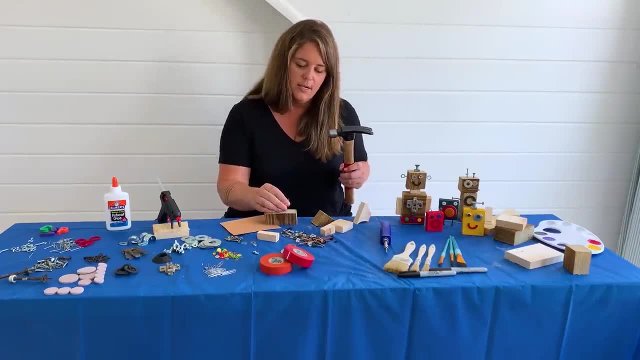 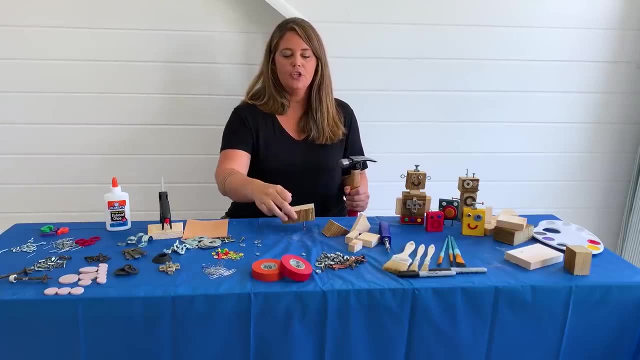 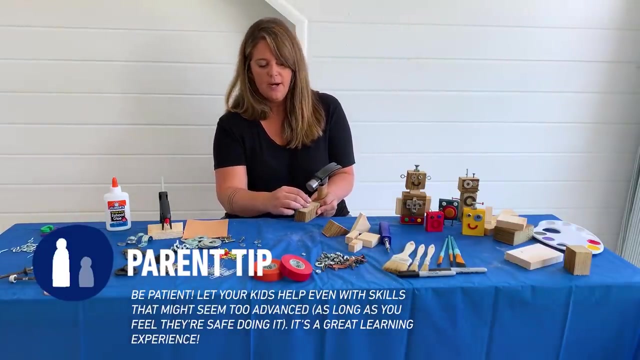 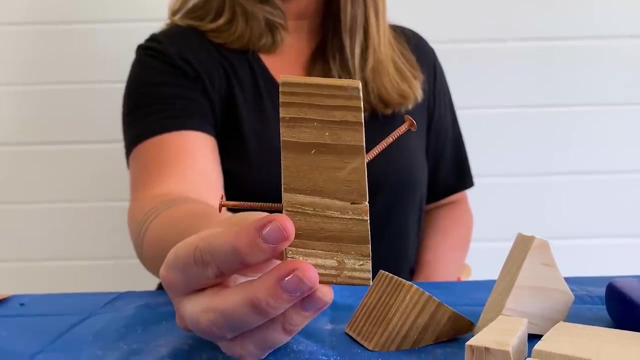 copper screws of my hammer and I'm just going to tap it right into the side. Now, when I'm attaching my second arm, it can be a little tricky because you can't really rest it. I found the trick is to pull one arm over the edge and hold your robot off the edge. What I love about this is that you can. 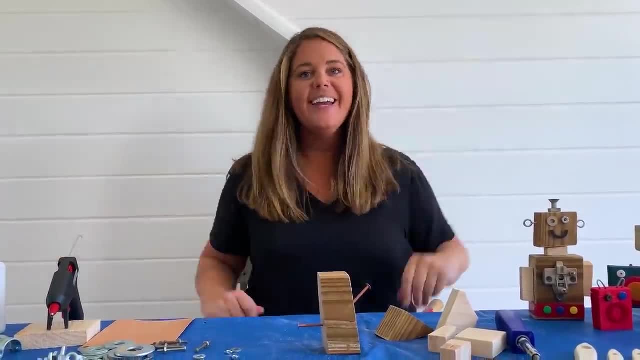 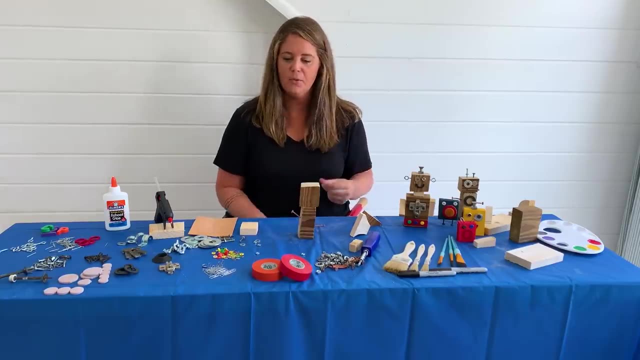 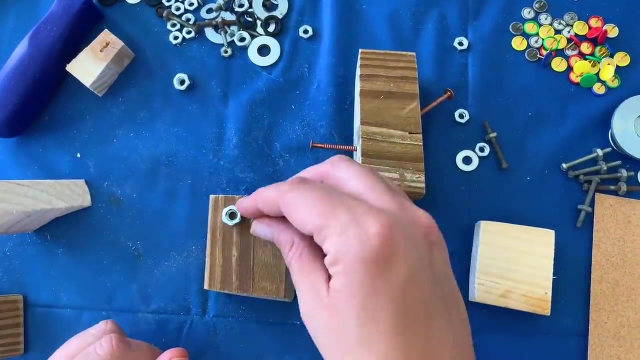 do this, or he's kind of like celebrating. Now I'm going to focus on my head And I'm actually going to go for like a really big kind of jumbo blockhead. look on this one. And again, it's just preference and having fun. I love the kind of mismatched eye look, So I'm going to use a nut. 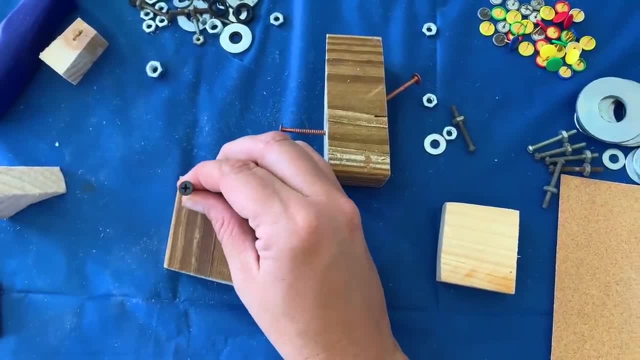 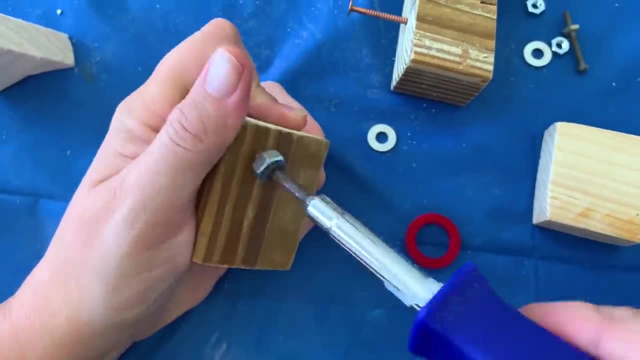 and washer combo. So I'm taking a screw. just a pro tip. If you tap the screw in a little bit, it makes it easy. So now for the washer. I'm just putting a little dab of hot glue on my fingers. 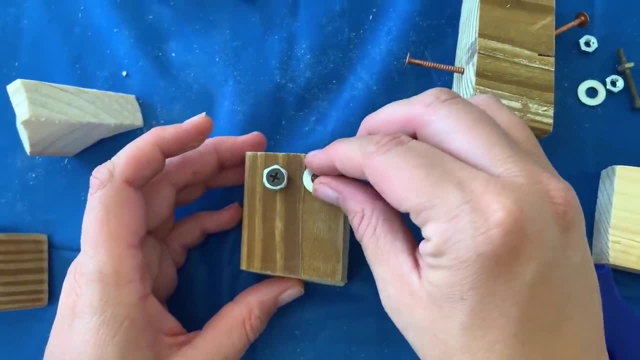 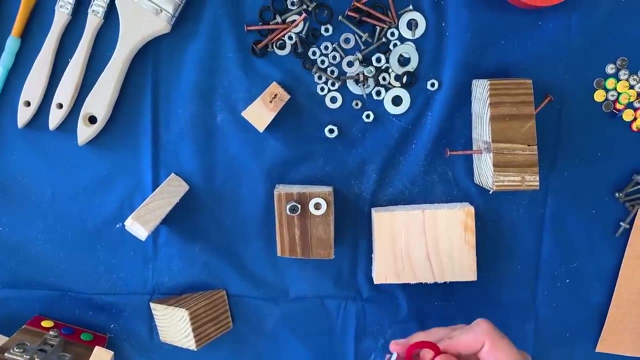 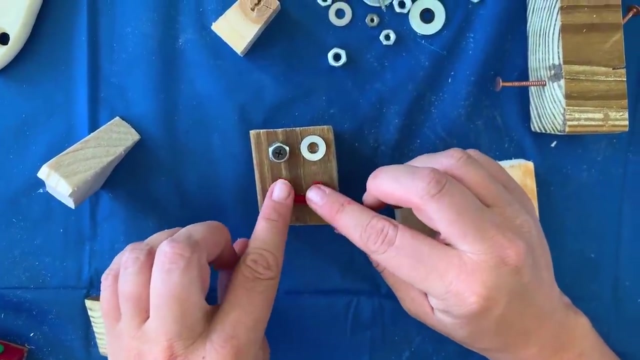 and then placing his eyeball For the mouth. here I found these little- I think they're from plumbing, like a plumbing piece here. I thought it made a perfect smile. a little bit of glue, Pop them on. I mean, come on, it's so cute. I gave this guy a little kind of 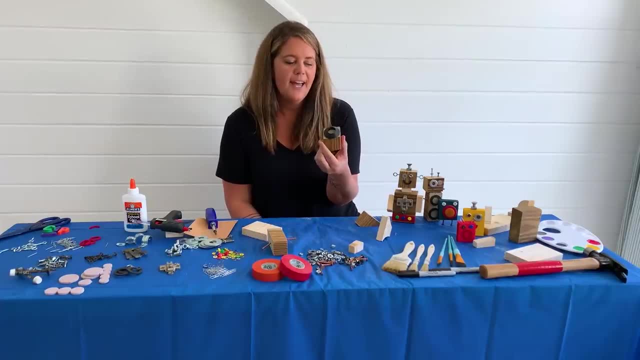 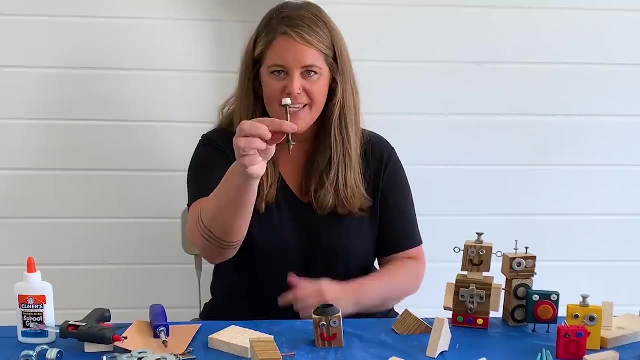 washer hat. He's looking super cute, but I think I want to take it next level. I found some extra. I think they're old doorstops in my garage And I think I'm going to put that into his hat. I'm 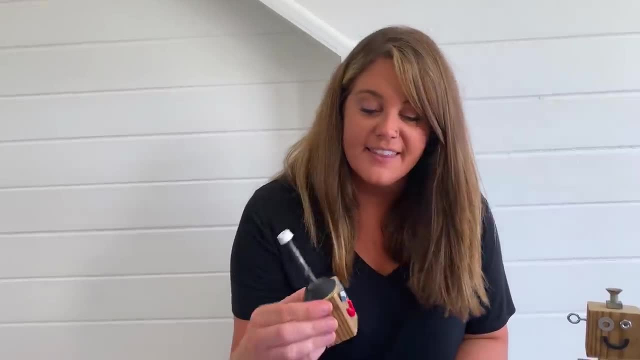 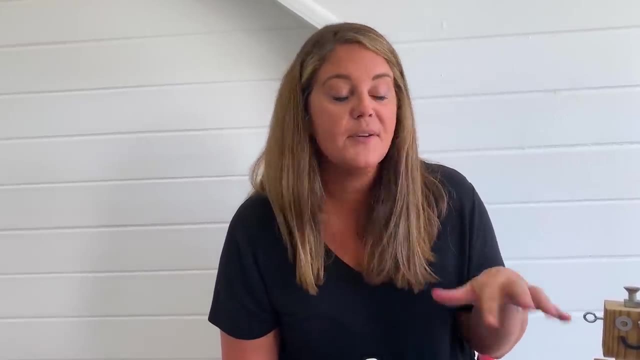 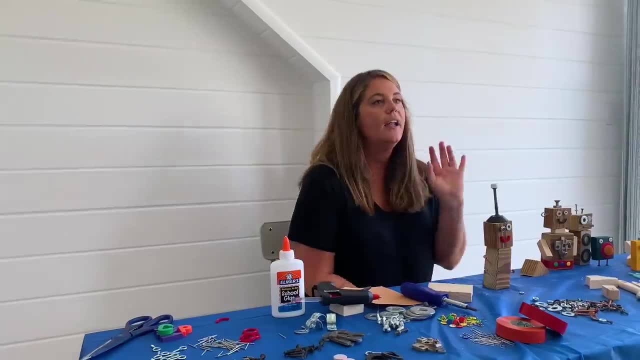 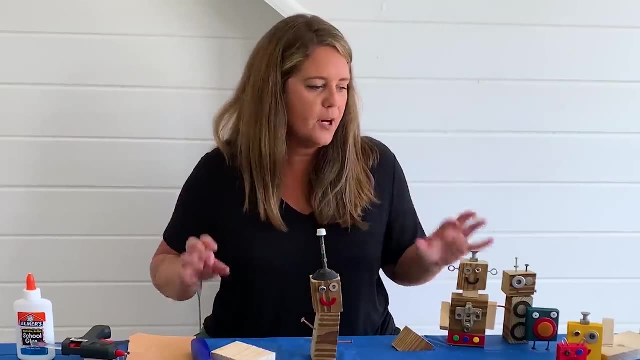 our body And then we have our body, And then we have our body And we're going to work on attaching those together in a minute And it's really important to mention here that we are clearly not going for perfection. This is a completely imperfect project. Tape is really great for kids. 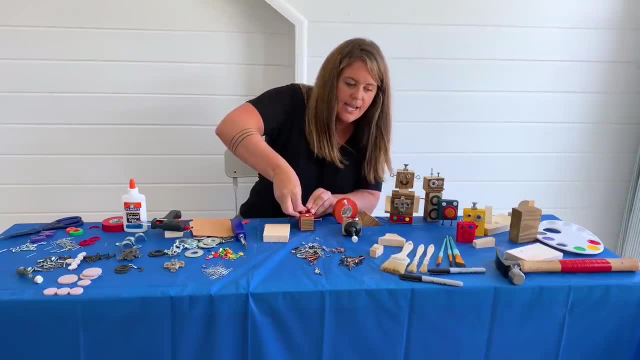 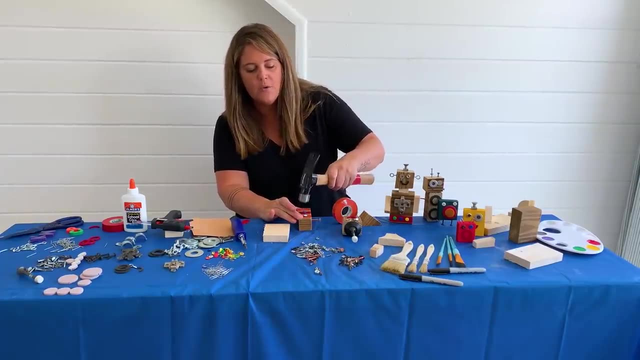 as an option for decorating, because it's very simple to use. I'm going to put a tack in here. I'm actually going to tap it down with my hammer because I am using pretty hard wood Works better, All right. so I'm really happy with his head and his trunk, but 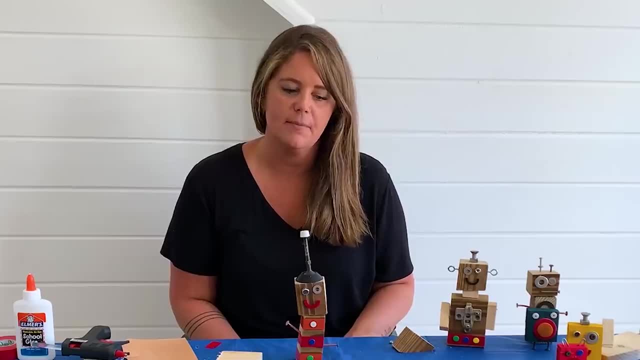 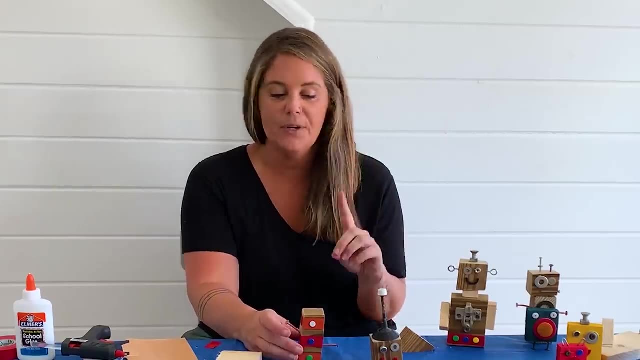 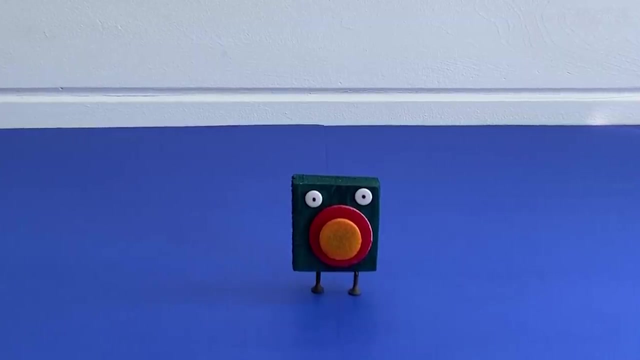 I do think the little guy needs some legs. He's feeling a little stubby to me right now. One thing that I learned kind of in my years of wooden robot making with my kids is that three legs are better than two. This guy here has two legs and he's working, but sometimes they can be a little bit. 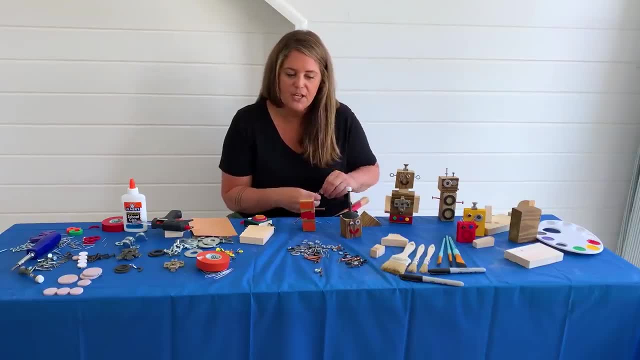 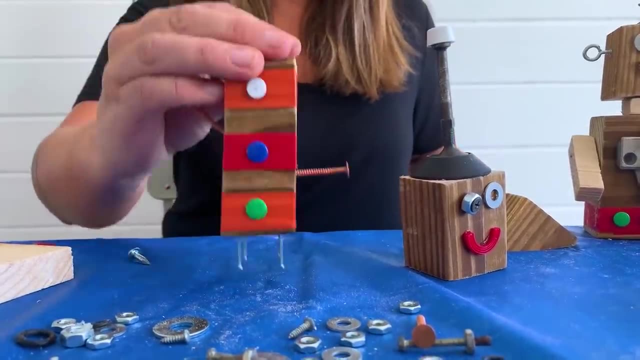 easier to fall over. For the legs here I'm just going to use a bunch of little finishing nails. I think that will be super cute, All right. so we have his body, We have his head. I'm just going to pop this on with a little bit of hot glue and then I'm going to talk. 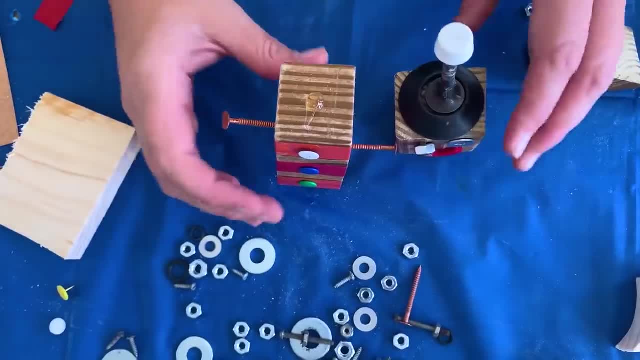 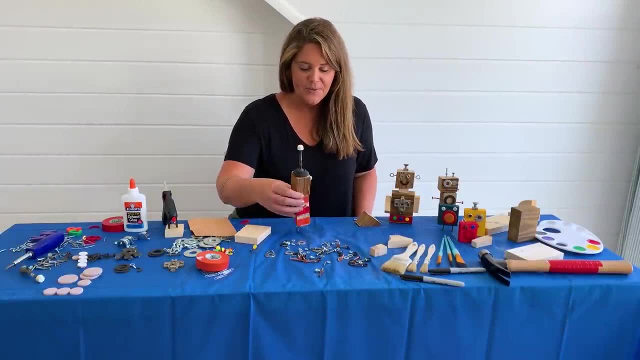 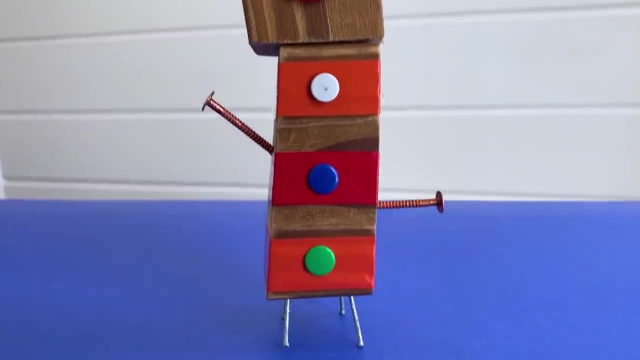 you through how I made some of the other robots, to just give you a few more ideas of how different things can be reimagined into various parts. All right, I reveal to you our little robot. Super cute, right? I just absolutely love these. This guy: again, we used nails for arms, We used 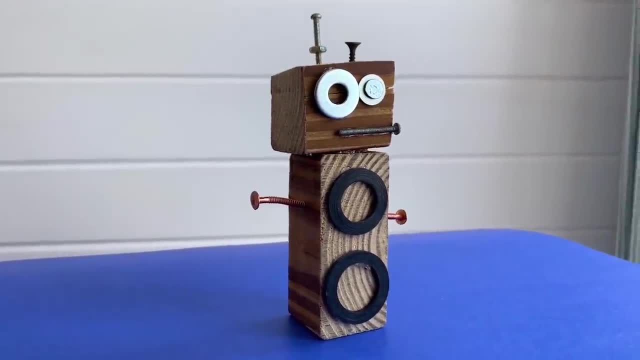 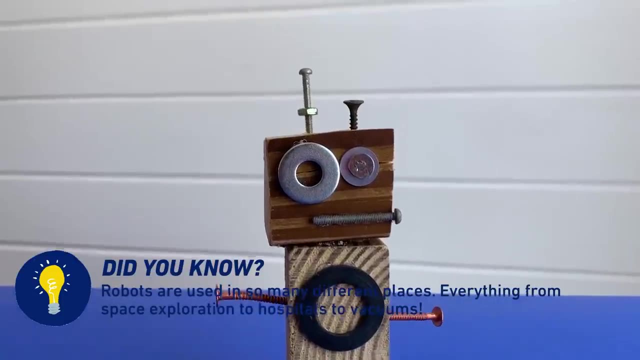 rubber washers here for his kind of trunk decoration, And then we used a variety of different screws and bolts and washers for all of his features. All right, and then for this little one here we have this like random hardware part that we had left in.